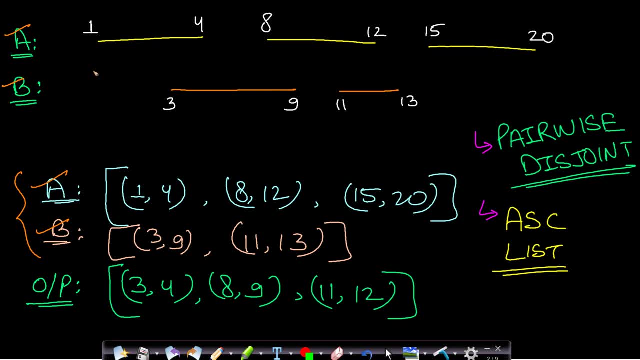 are already mentioned here. Now I have diagrammatically represented them so that it becomes easier for you to understand. Now the list a is having three intervals and list b is having two intervals. Now we need to return all the intersecting intervals, So in this case you can. 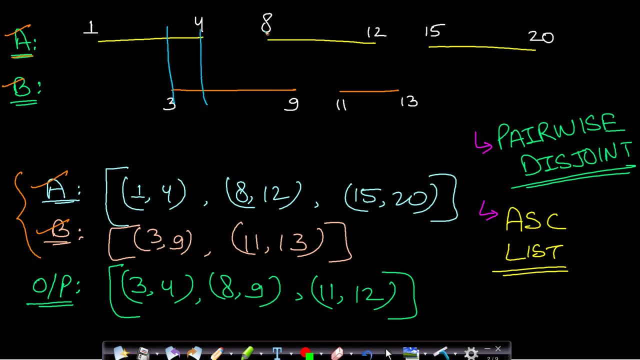 see that the intersecting intervals are from 3 to 4 and from 8 to 9 and also from 11 to 12.. So these three intervals are from 3 to 4 and from 8 to 9 and also from 11 to 12.. So these three 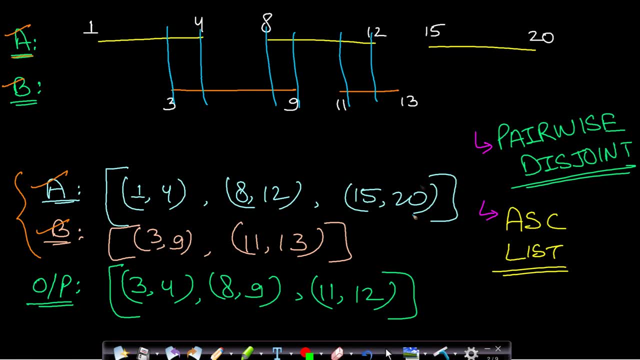 intervals should be included in a vector, that means in an array, and should be returned. So I have included all three intervals- 3 to 4,, 8 to 9 and 11 to 12, and we will have to return it Now. they have also mentioned about some important conditions. The first condition is that if we have 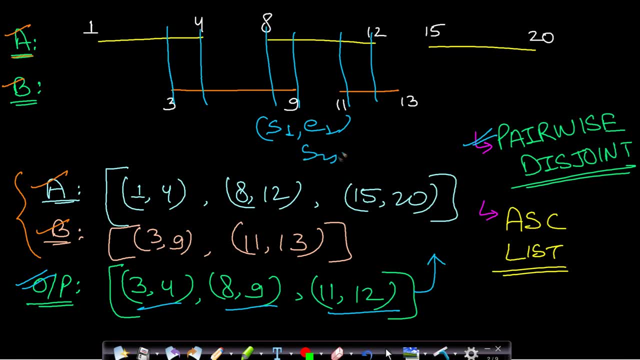 two intervals, s1 comma e1 and we have s2 comma e2. then there is no such pair, s1 comma e1 and s2 comma e2, where s1 is equals to s2 and e1 is equals to e2. So we have to return the intersection. 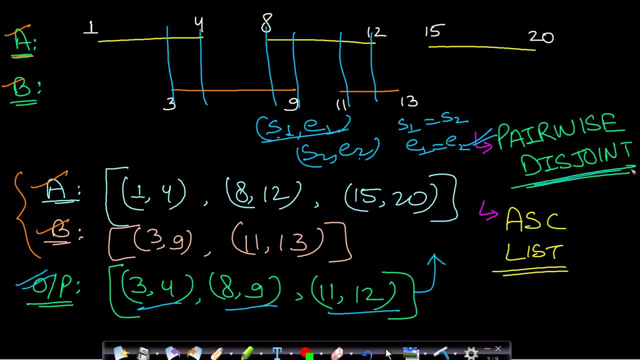 s1 comma e1 and s2 comma e2, where s2 comma e1 is equals to e2. That means all the pairs are disjoint. That is, no two intervals are exactly the same in a list. And the second condition says that all the lists are in increasing order, that means in ascending order. So if the list were not present, 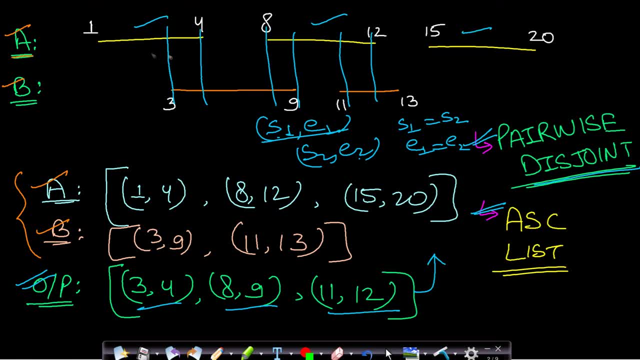 in ascending order, then we would have to sort it in ascending order in order to solve this problem. Okay, Therefore, since it is already given, so we do not need to sort the intervals. So I hope you got the problem statement clearly now. So let us now see how do we solve this problem. 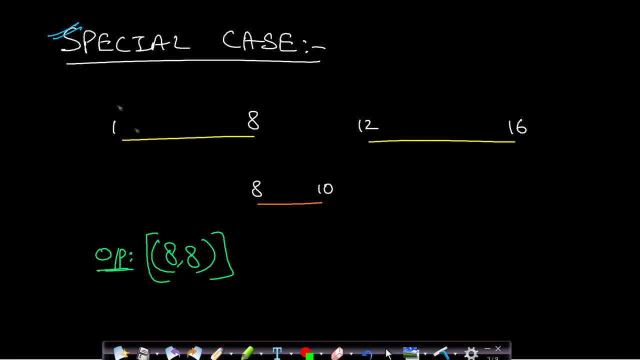 Now, before going to the solution, we will see the special case. In this case you can see that the first interval is from 1 to 8. second interval is from 12 to 16.. In the second list we have only one interval, from 8 to 10.. In this case you can see that there is no overlapping, but only at one. 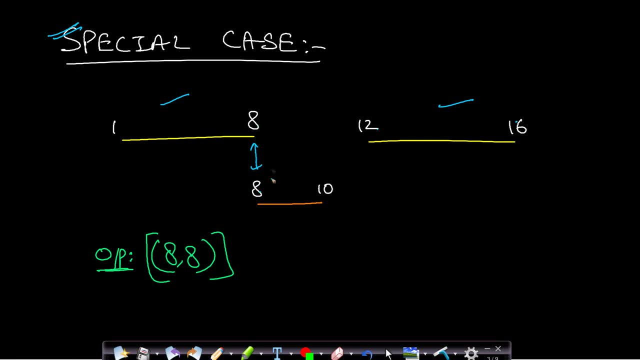 point. So if there is overlapping at only one point, then the starting and ending point will be same. So we will have to include 8 comma 8 in our output. So this is one special case for this problem. Now let us look at the different possibilities. So let us look at the different. 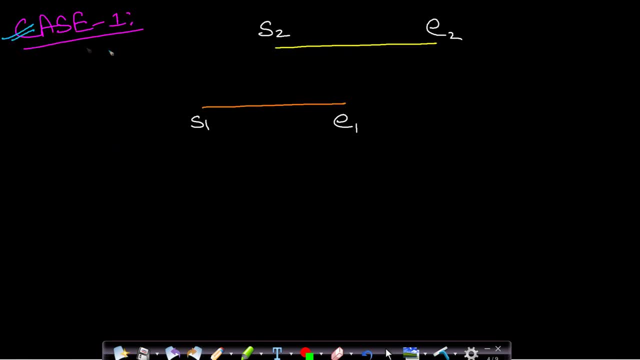 possible cases in order to solve this problem. So the first case is like this: You are given an interval s2 comma e2 in list 1 and an interval in list 2 as s1 comma e1.. Now how do you find if? 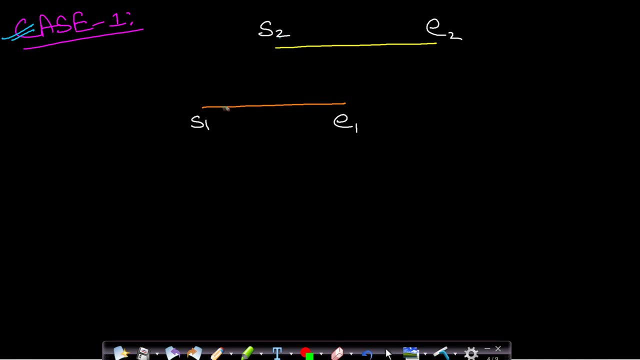 these two intervals are intersecting, So in order to do it, you need to check this s1 with e2.. So s1 should be less than equals to e2 and also e1 should be greater than equals to s2.. If this is, 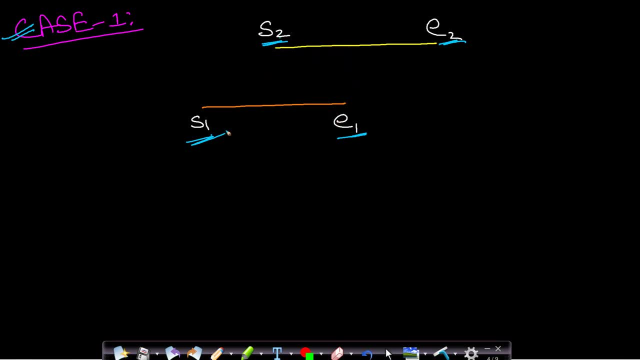 true, then we can say that there is some intersection somewhere. So in this case, you can see that s1 is less than e2 and e1 is greater than s2.. Therefore, there is an intersection. Now let us look at case 2.. In this case- 2, we will follow the same method. 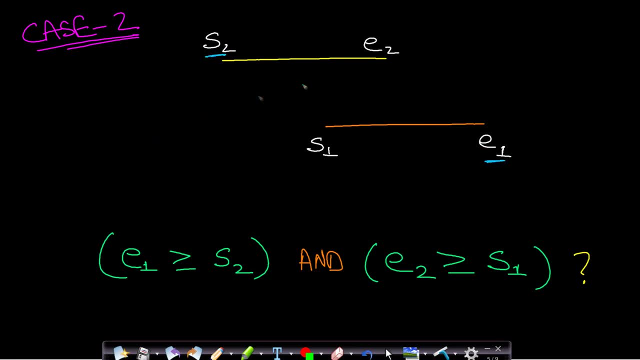 If e1 is greater than equals to s2 and e2 is greater than equals to s1, then there will be some intersection in between. I have already written the condition here, So you can see that e1 is greater than equals to s2.. Okay, this is correct, But now we need to see the intersection. 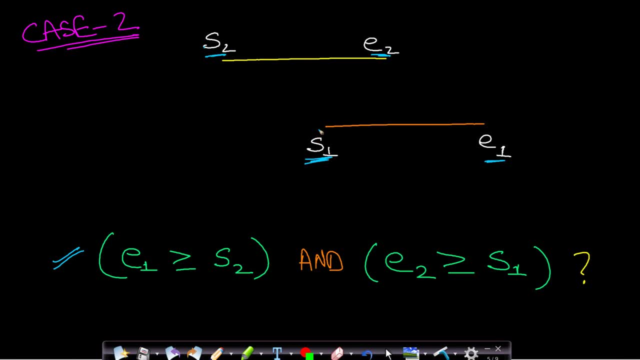 See if e2 is also greater than equals to s1.. So this is also correct. Therefore, there must be some intersection in between. Now let us look at case 3.. In this case 3, we will do the same thing. We. 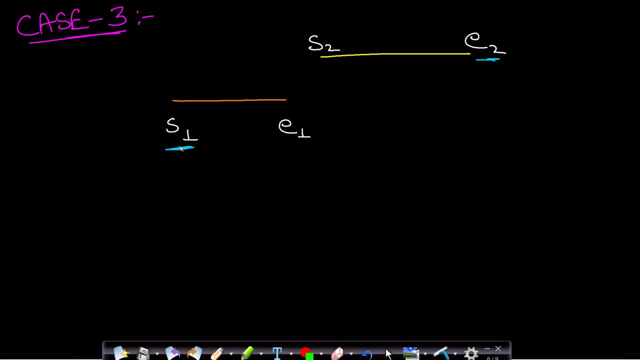 will check if s1 is less than equals to e2.. Yes, s1 is less than equals to e2.. Now we need to check if e1 is greater than equals to s2.. And why are we doing this? Because we need to also check that. 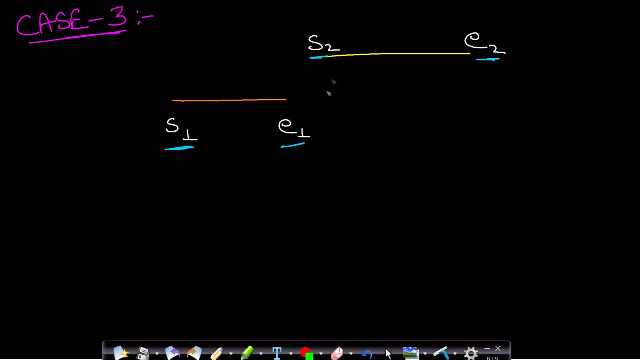 if s1 is less than equals to e2, then e1 should be greater than equals to s2. So that there is some intersecting part, But e1 clearly is less than s2. Therefore they are out of bounds and there is no intersection in this case. Now, if you look at this case 4, then we will do the. 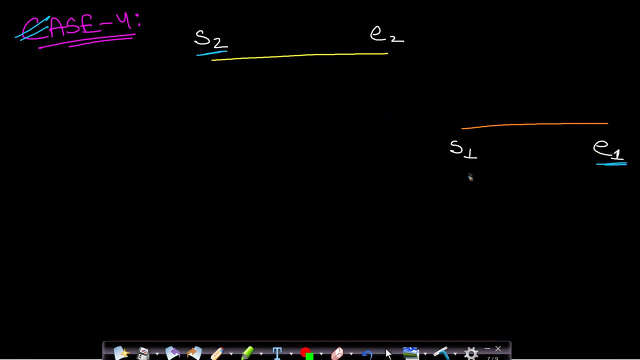 similar check, e1 is greater than equals to s2 and s1 should be less than equals to e2.. Or you can say that e2 should be greater than equals to s1. But this is not true. Therefore, there will be no. 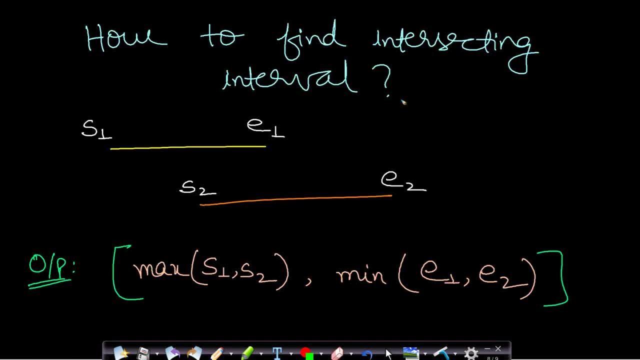 intersection. Now how to find the intersecting interval. So let us say we are given two intervals to e2.. So how do you find what is the range of intersection? So in this case, what we will do is first we will have to determine whether they are intersecting or not. In order to do it, e2 should. 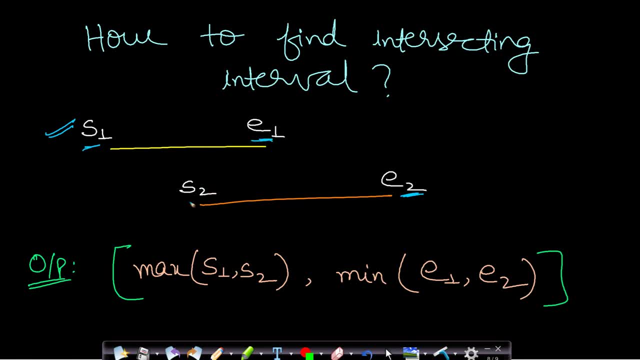 be greater than equals to s1 and e1 should be greater than equals to s2.. If this is true, then they are intersecting. So first of all, we will need to find whether they are intersecting or not. So if you find that they are intersecting, then the second thing is to find in what interval in 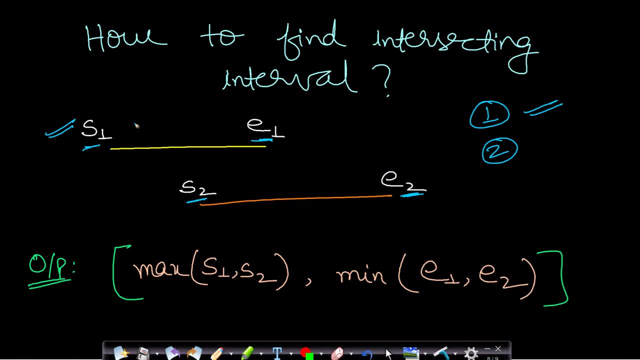 which they are intersecting. So, in order to do it, you will have to take the maximum of s1, s2 and the minimum of e1, e2.. So the maximum of s1, s2 is s2.. So you will draw a line here And the minimum 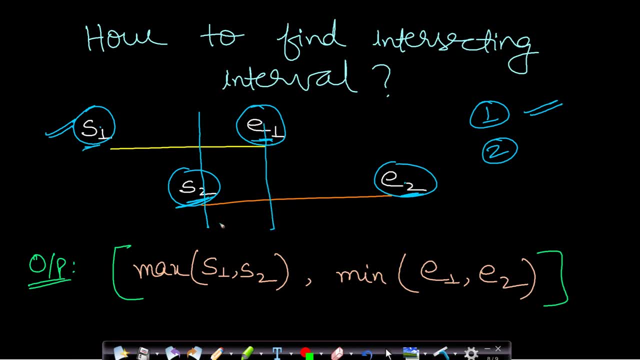 of e1, e2 is e1. So you will draw a line here. So this is your intersecting interval. So I hope this is a very simple concept And just by drawing some diagrams on your notebook you will be able to understand how I did it. So this will be our output. 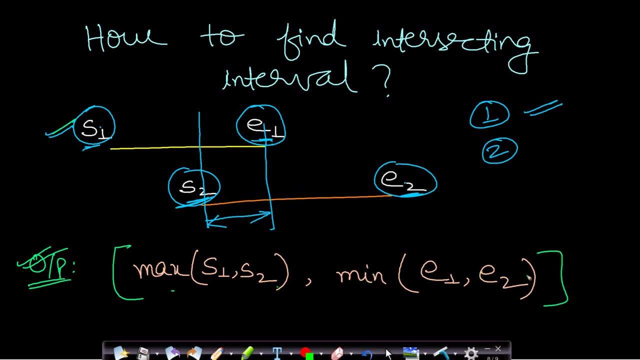 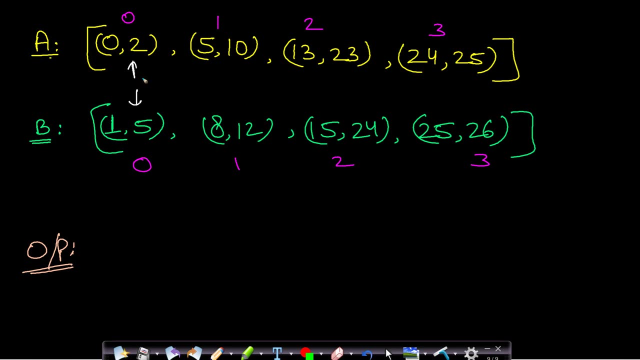 So in this case, what I will do is, since we are given two lists, a and b, and we need to output all the interval points, So I will take a- a pointer, a ptr and a- b pointer, b ptr And I will keep incrementing it. And where do you stop? we will stop if a ptr goes out of bounds or b ptr. 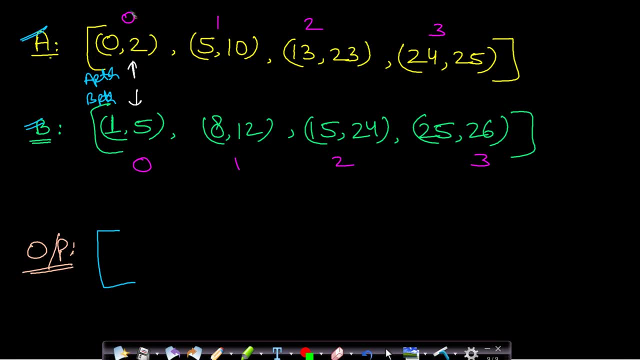 goes out of bounds. Okay, so we are starting at this point: index zero for a and index zero for b. Now, in this case, we will apply the same condition we learned in the four cases, So the first value of b should be less than equals to the second value of a, And the second value of b should be: 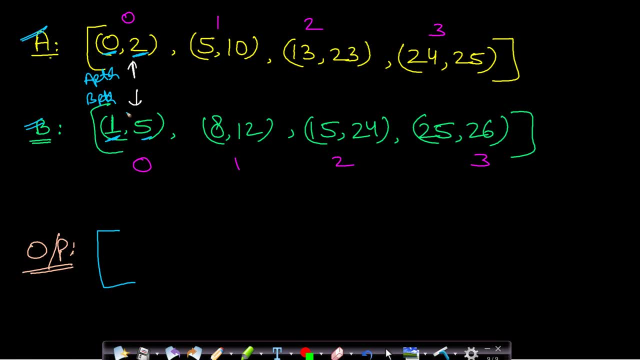 greater than equals to the first value of a. This is true, then we will have an intersection. So in this case, it is true. Now, how do you find the intersection? Now, in order to find the intersection, we will have to take maximum of. 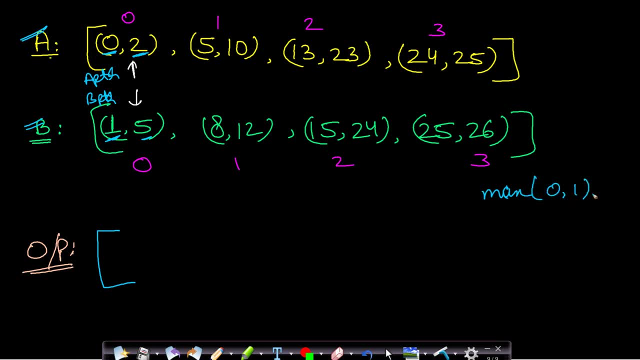 zero comma one, which is the first value comma, minimum of the second values, which is two comma five. So this will come out to be: maximum of zero comma one is one. minimum of two comma five is two, So one comma two. so we will have to push this one comma two in our output vector. 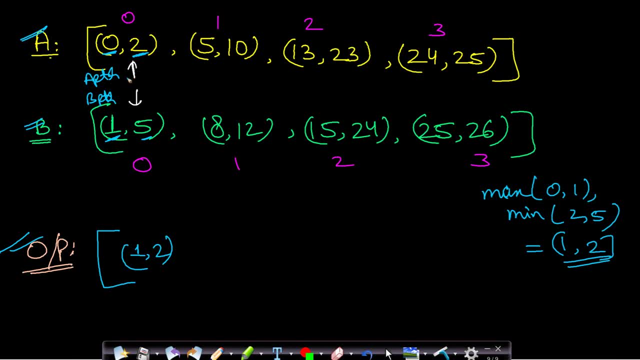 Now, since we have found the intersecting interval, so we will have to increment the a pointer or b pointer or both. So how do we increment it? Now? you will have to increment based on the second value. So the second value of this, a ptr, is having value two and the second value of b ptr is having 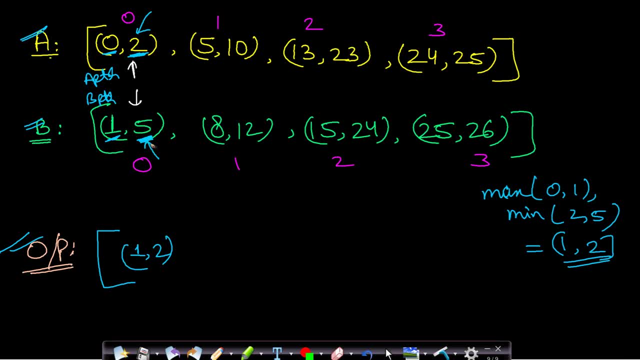 a value five. So the span of b ptr, the current value, is more than the span of this a ptr value. Now, since the range for this point is going to five and this point is just going to two, so we will have to increment this a ptr value because the b ptr value is having a higher span. 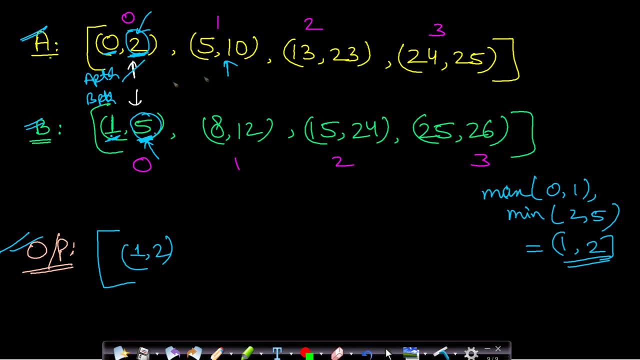 So it is very logical to just increase a ptr value Now. a ptr value is pointing to index one. Now we will again do the same process. So if we repeat the process then we will have to again check if one is less than equals to 10.. And five is greater than equals to five. So this is true. 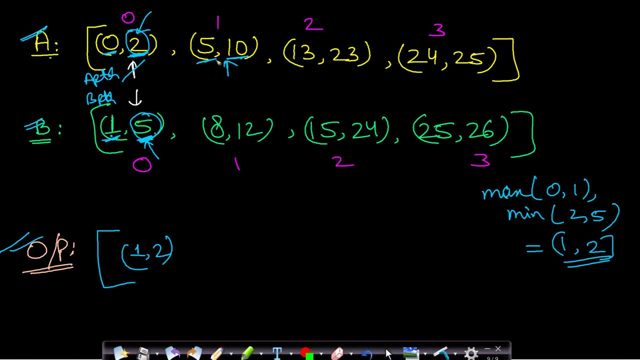 Therefore we will have an overlap. So what will be the overlapping point? we will again use the same formula which we had used: maximum of the first values. So first value is five, one, five, one, five for this one and one for this one. 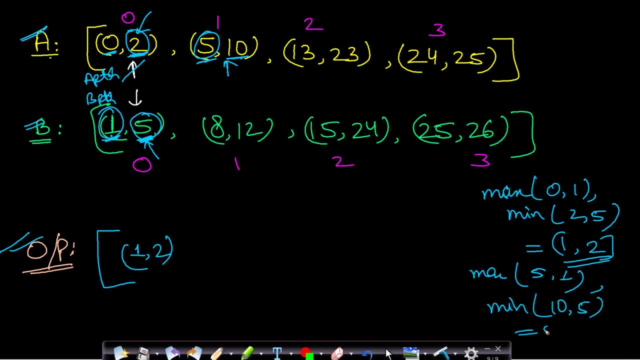 minimum of the second values. So 10, five. so this will come out to be five, five. okay, now, this is just a single point. So five, five will get inserted. now, which pointer to increment? Now we can see that the b pointer is having a span till five. 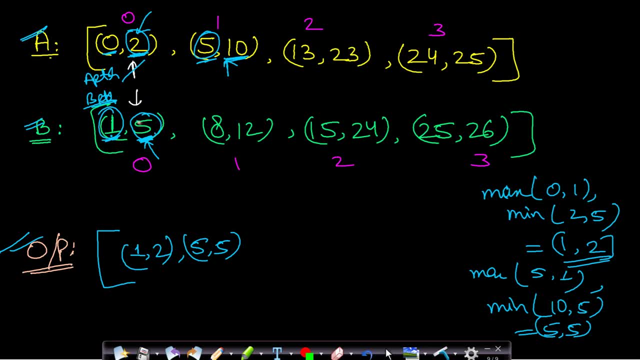 and a point a span till 10. so b pointer is having a lower span. so b pointer will be incremented to the next value. now, similarly, we will keep repeating the process. in this case 8 is less than 10 and 12 is greater than 5. so there is an intersection and what will be the intersection point maximum of 5 comma 8? 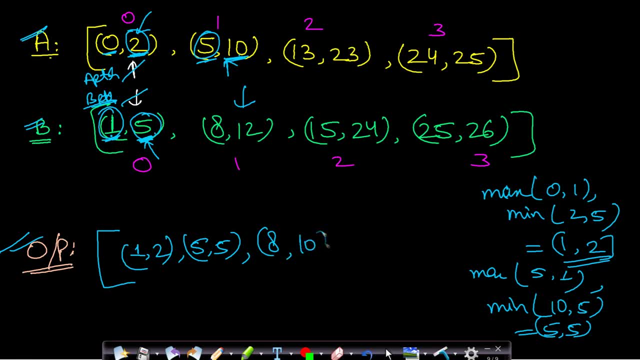 which will be 8, and minimum of 10 comma 12, which will be 10. okay, now which one to move? we will move this a pointer, because 10 is less than 12, so this 10 is having a lower span, so a pointer will be. 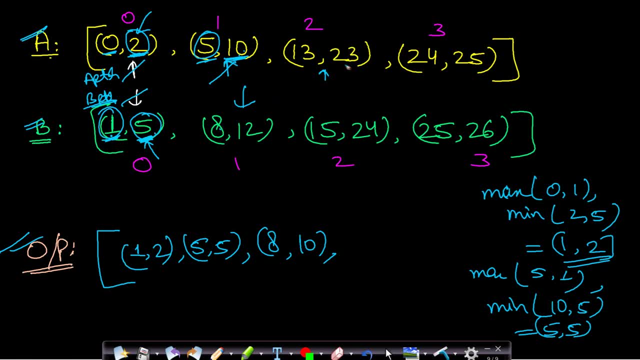 incremented now. in this case, 8 is less than equals to 23, but 12 is also less than 13, so this is having no intersection. so if there is no intersection now, we will increment based on second value. so 12 is less than 23, so we will have to increment this b pointer now. again, we check for intersection. 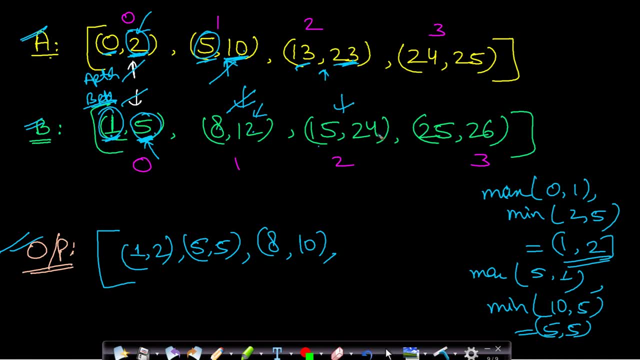 and 15 is less than equals to 23, so b pointer will be: 29 by 10 equals to 7альное person of the first other群, and 24 is greater than equals to 13so this is true and the intersection point will bemaximum of the first. 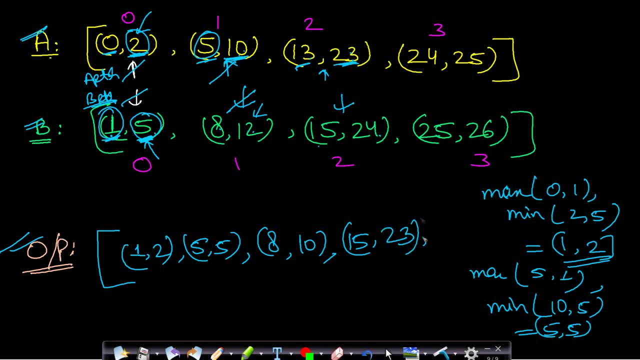 values 13 comma 15, which will be 15and the minimum of the second values, 23 comma 24, which will be 23.. now again we will increment a pointer, because 23 is less than 24. now again we will check of 15 is less than equals 25. 24 is also greater than equals to 24, so there is an intersection and you 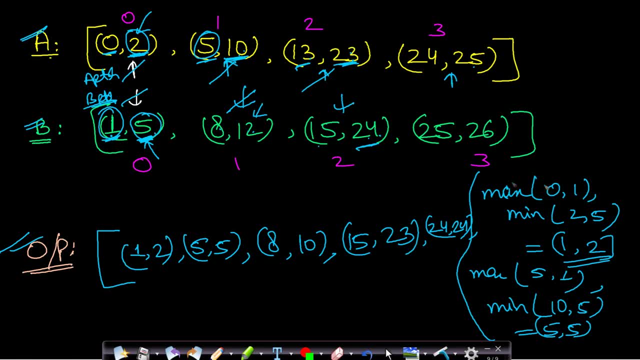 section point is 24 comma 24, so you will have to use the formula. actually now 24 is having a lower span, so this will get incremented, since 24 is less than 25. now you will again check. you can see that 26 is greater than equals to 24 and 25 is less than equals to 25, so there is an intersection. 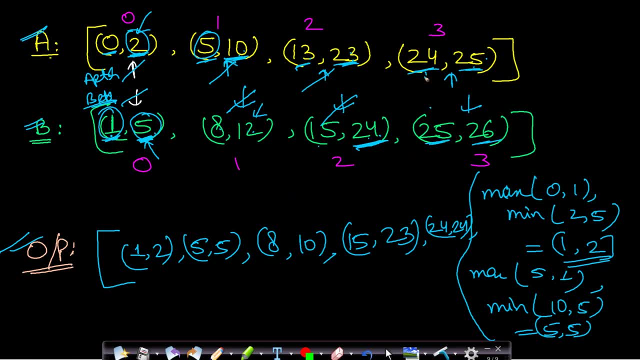 and what will be the intersection point. it will be maximum of the first values, 24 comma 25, which will be 25, and a minimum of the second value, 25 comma 26, which will also be 25. so the next step is to increment the pointer. so a pointer will get incremented and it will go out of bounds. 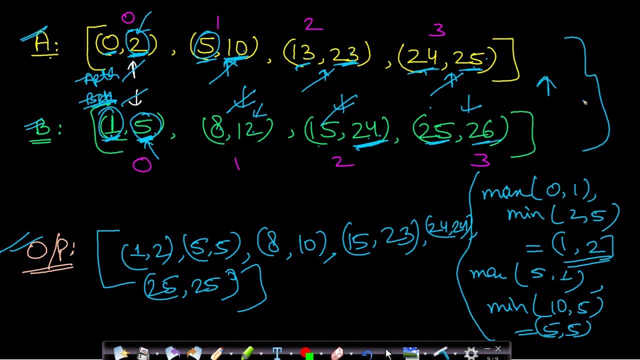 now, if any of the a pointer or b pointer goes out of bounds, we will stop there and whatever is in our output list, we will have to just return it as our answer. so these are all the intersection intervals. so i hope you were able to understand this. now the time complexity for this will also 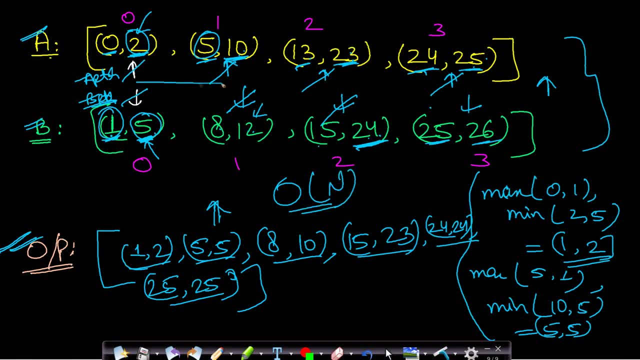 be o? n, since we are just traversing. each of this gives us a minimum of the second value, followed by a minimum of the second value, which will be 25, and the minimum of the second value, 25, which will also gives us a minimum of the second values'. 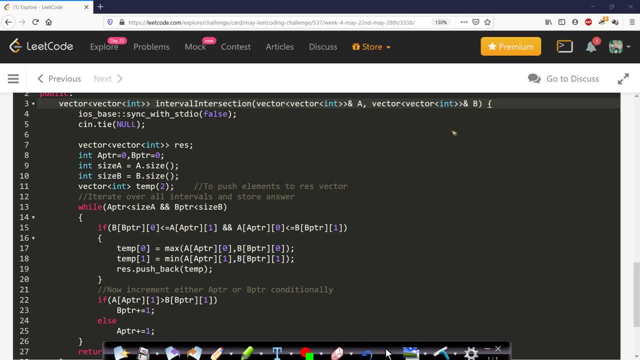 only once, okay, so let us now look at the code. now in this problem, we were given to list a and b and then i took a resultant list where i will store the result, and i have taken a aptr and bptr for pointing to the first values of both the list in order to process the list now i have also taken